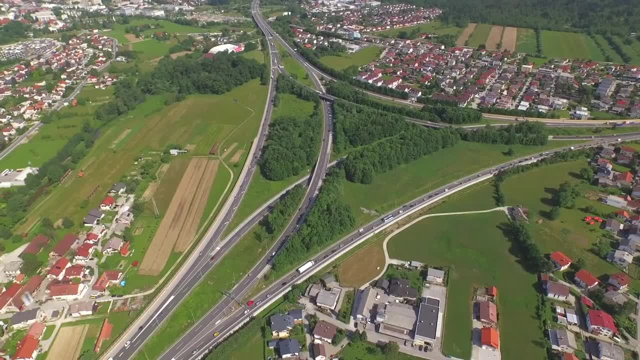 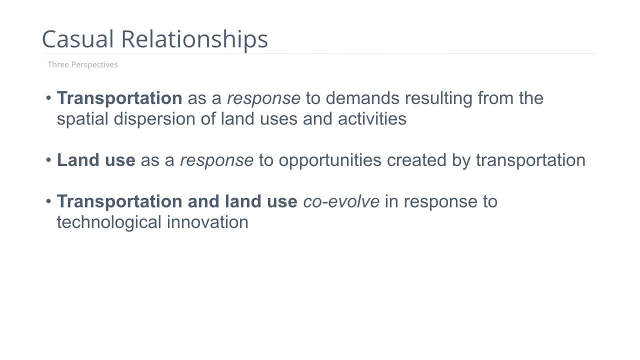 created by transportation systems, such as the development of the interstate highway system, enabling the development of residential suburbs. A third view is that transportation and land use co-evolve, and co-evolve in response to technological innovation and will trace the transition of new technology in transportation and how it affected transportation and land use. 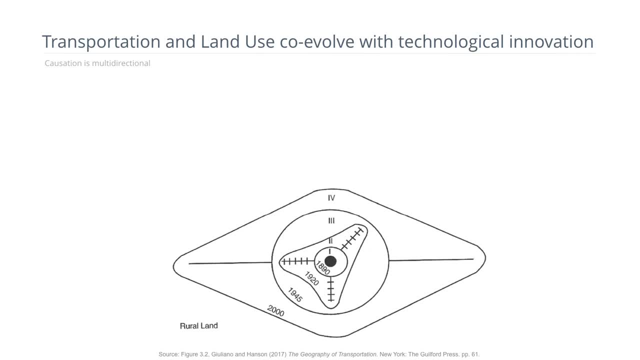 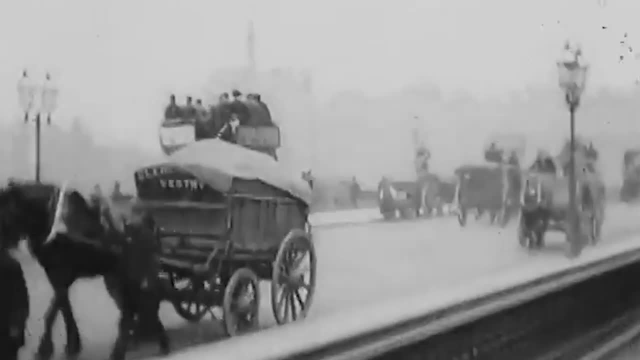 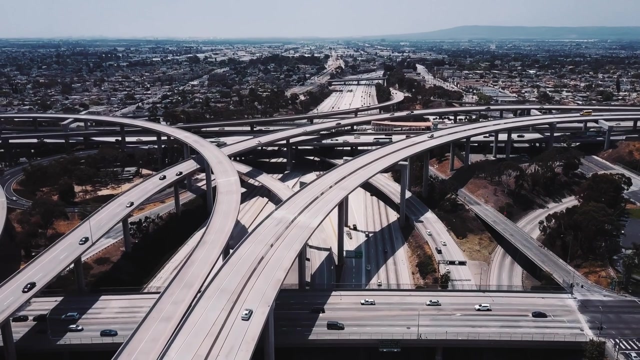 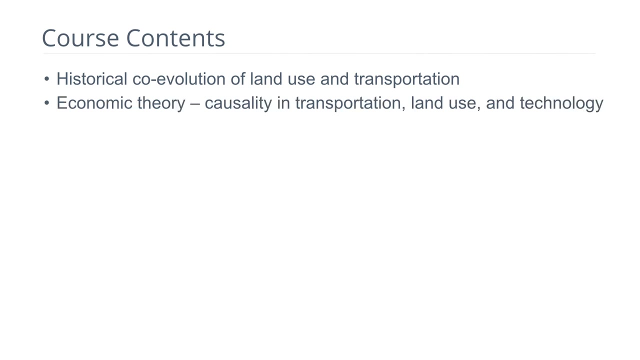 This diagram gives a preview of what we'll be talking about as how, and showing how cities have evolved from essentially relying on human power and animal powered transportation, which was very slow, to the current era of automobile transportation. The course contents are as follows: we'll discuss the historical co evolution of Land-Use and Transportation Systems. 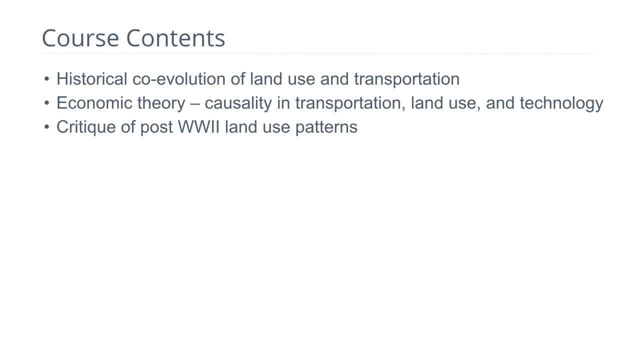 We'll explore some economic theory. we'll critique the post-World War Two land use patterns that have emerged and then explore some strategies in Land-Use Planning and strategies and transportation planning that can address the interaction of land use and transportation Towards the end of 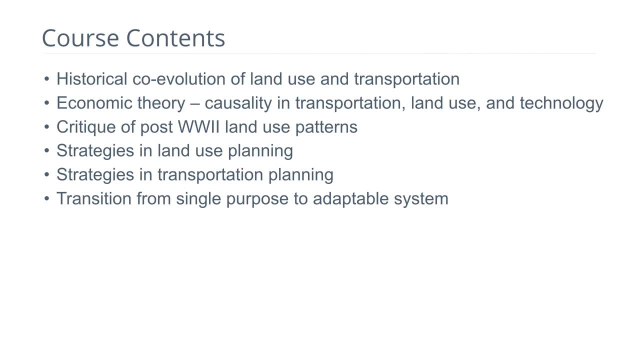 the class, we'll explore the transition from single purpose systems both in land use and transportation and in Energy. at home you can see these changes. Please watch your project. talk about land use and transportation when filling places around perché ankemel? Vitamin N, adaptable systems. And finally, we'll conclude with a discussion of the future. 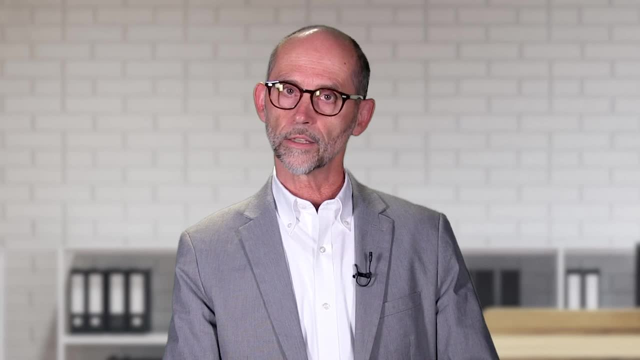 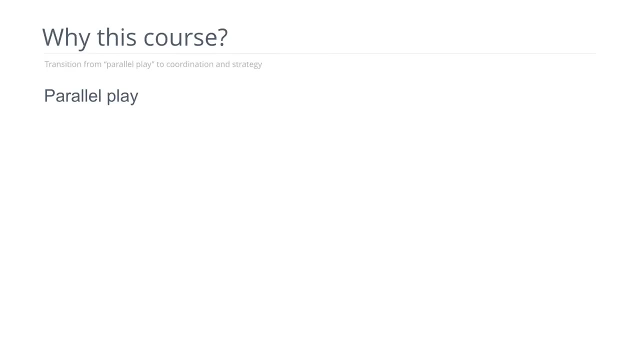 of land use and transportation relationships. Why this course? I think we're in a historical change from a way of looking at land use and transportation as parallel play- the idea of kindergarteners are playing beside each other but not with each other, and parallel play is how we used to do land. 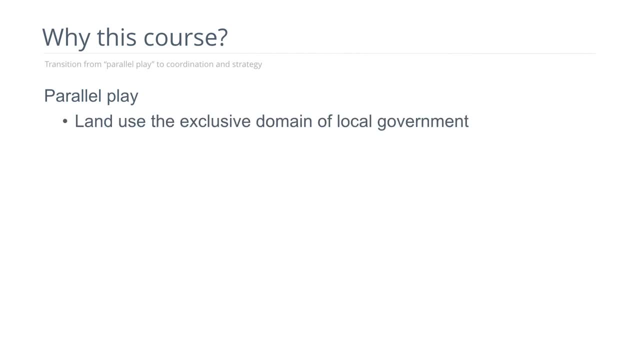 use and transportation planning. Land use was the exclusive domain of local government and zoning generally followed market demands. Transportation was more a top-down endeavor, influenced by federal, state, regional and county initiatives, and the two realms were not closely coordinated. Now we're trying to 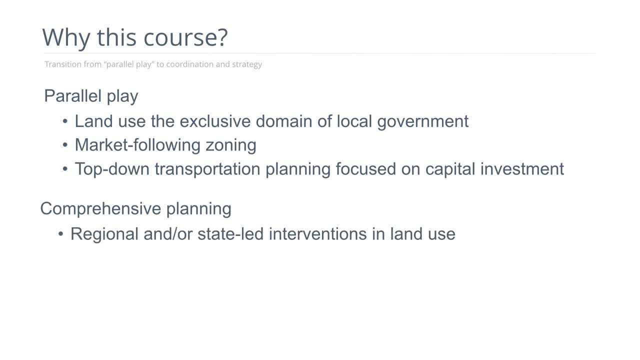 be more comprehensive about these two realms, and what we can see is regional and state interventions in land use regulation, more proactive zoning and requirements for coordinated strategies between land use and transportation. So let's begin you.